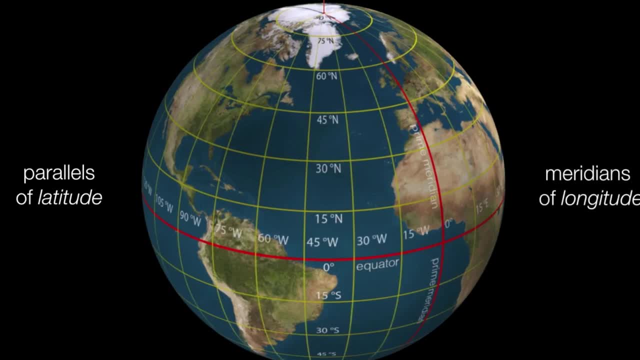 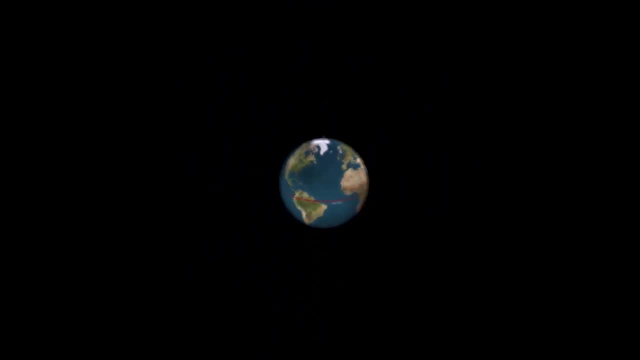 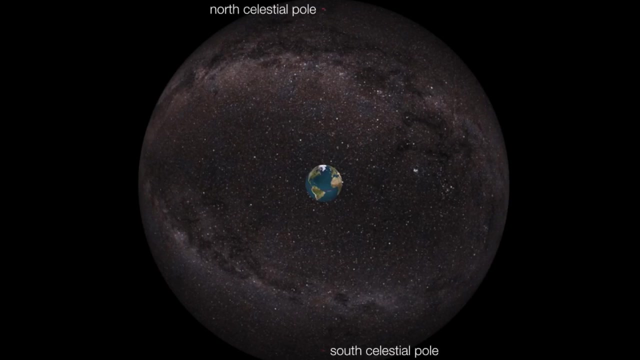 at in this video. We need to imagine the Earth is surrounded by a giant glass ball and onto which we're going to project our equator and our poles and any other lines that we might find useful. So here's our celestial pole, and the stars are painted on this glass ball as we see them. 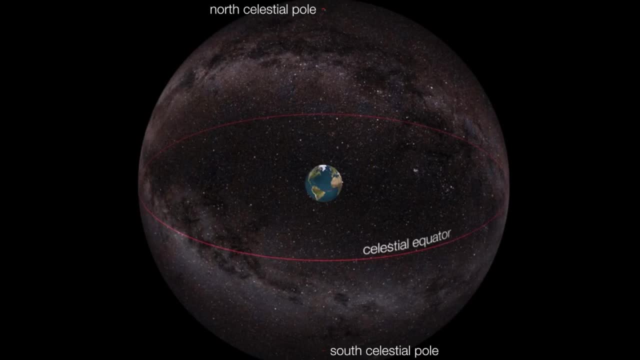 on the Earth And we're going to imagine the Earth is still and it's the rest of space that's rotating around us. And to do that we need a few bits of vocabulary, And the ones that I want to look at in this video is the word zenith and the word nadir or nader. 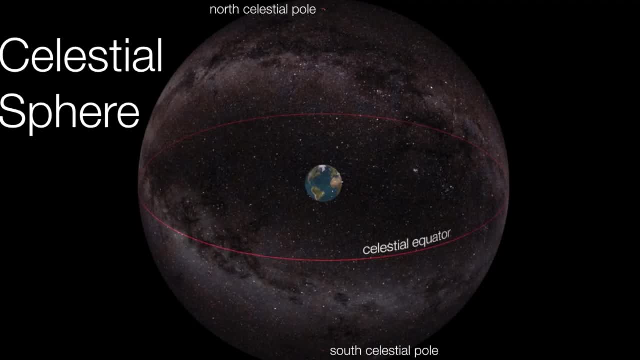 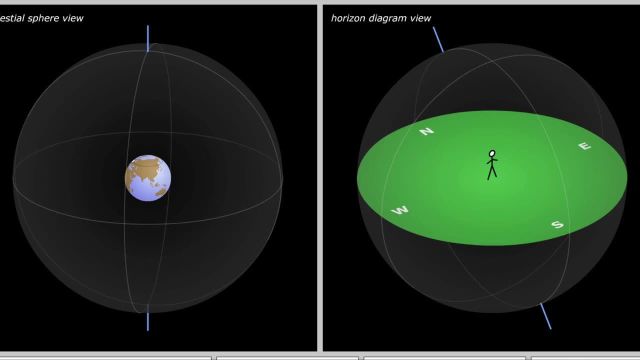 Okay, And so to do that, we're going to use this word, zenith, and the word nadir or nader, And we're going to compare views, One from the celestial sphere point of view on my left, and the one on the right is the observer's perspective. You'll notice. 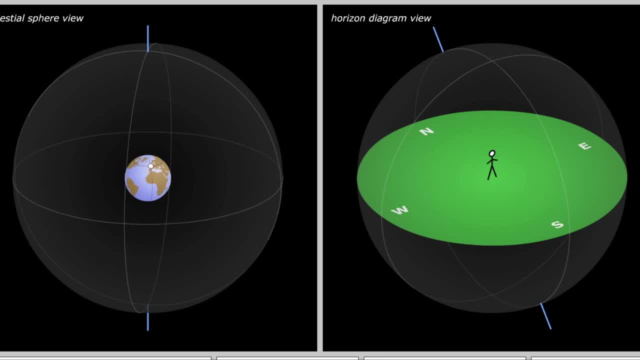 that I'm using this white dot on Earth which has started to rotate, and that's at battle. So there's you, the observer. directly above you is a point called the zenith, and that's unique to you. wherever you move, your zenith moves with you. it's. 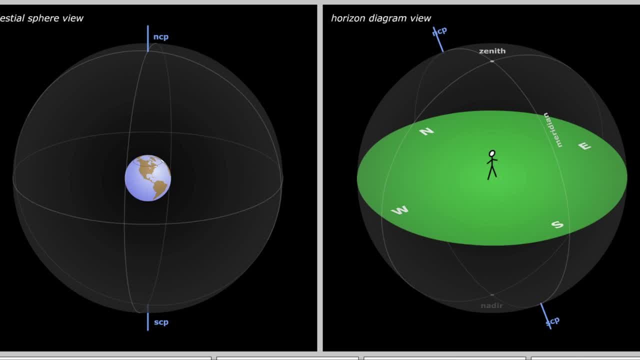 directly above your head on the celestial sphere and if you look, if you look at your feet and you go through the earth with x-ray vision on the celestial sphere, is the Nader or Nader? and I'm also going to mark on a possible path for the Sun. this would be called an ecliptic. 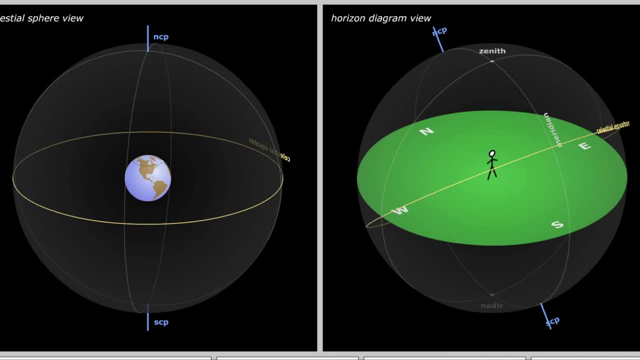 this line it's. you can think of it as the apparent path that the Sun takes on the celestial sphere and observe from Earth. So we're going to go for an eclectic view. So we're going to go for an ecliptic view. So we're going to go for an ecliptic view. 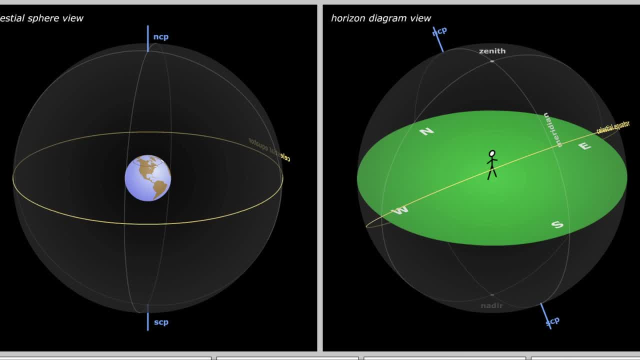 So we're going to go for an eclectic view. we've looked at the three bits of vocabulary that are going to help us use this celestial sphere and, to get started, we're going to look at three different star constellations. Perhaps the first one we should look at and hopefully recognise is Orion. So there it is, on the left, you can see.